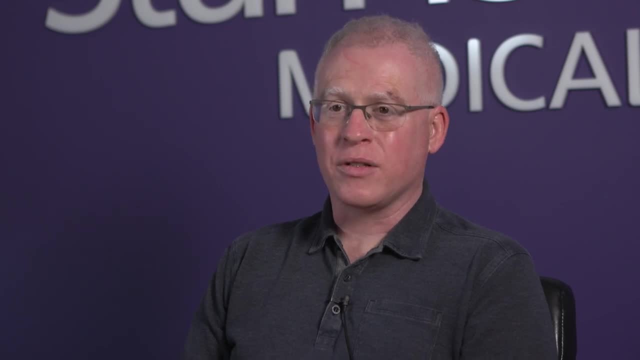 to remember that the universe is much cleverer than me, And so if I'm getting a result that I'm not expecting when I'm in the lab, it's not that the experiment isn't working, that the test is broken, it's that I haven't been clever enough. 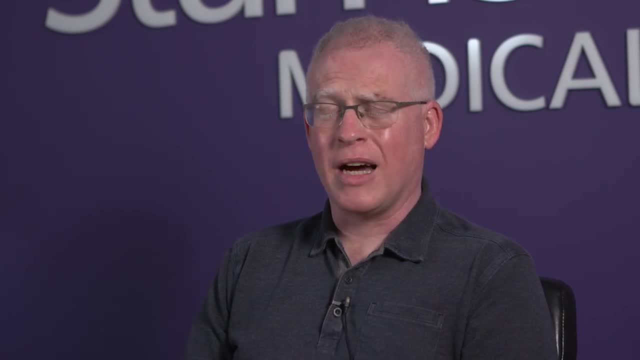 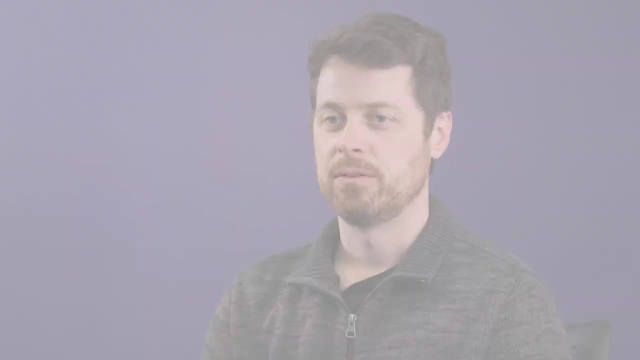 to think about what it's actually measuring. But keeping that in mind, usually you can get to the root cause of unexpected results a lot faster and maybe learn something along the way. My name is Ryan Field. I'm an optical engineer here at Starfish for the last couple years Before coming here. I have a background. 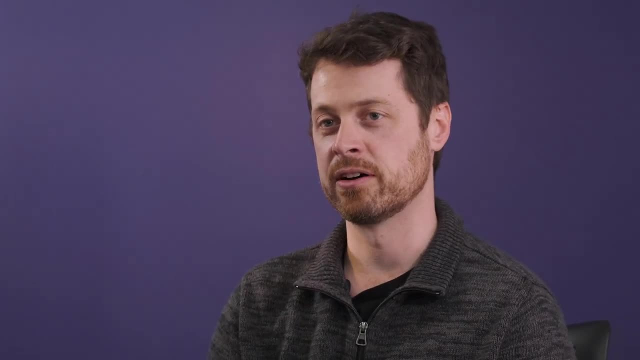 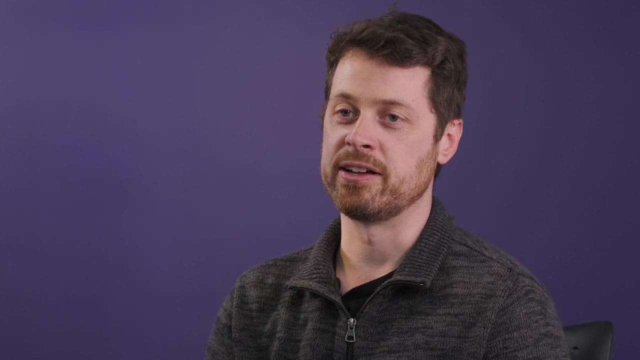 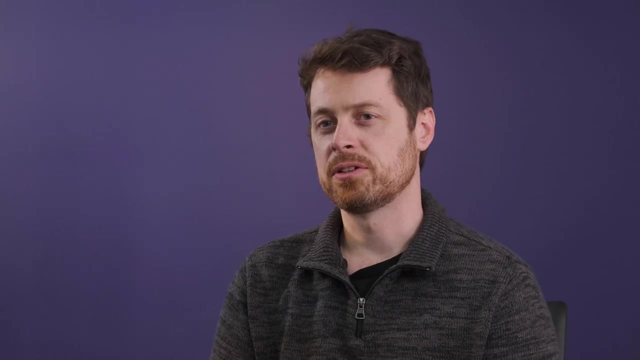 in ultrafast laser spectroscopy, which is a method of measuring changes in the optical properties and materials on very short time scales, And I also did some work working with surgical laser systems and surgical microscopes, Optical breadboarding, which is basically taking our optical system or subsystem and 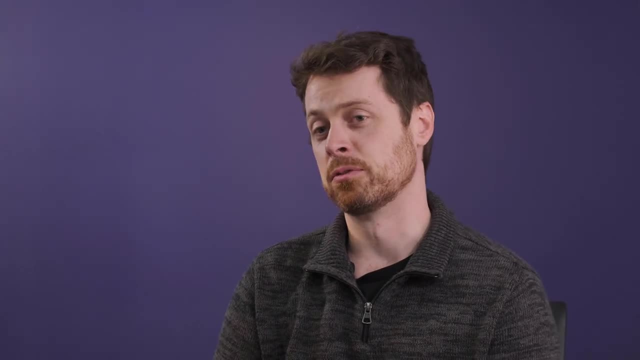 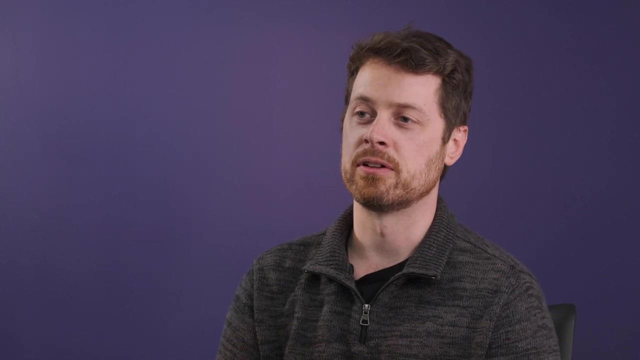 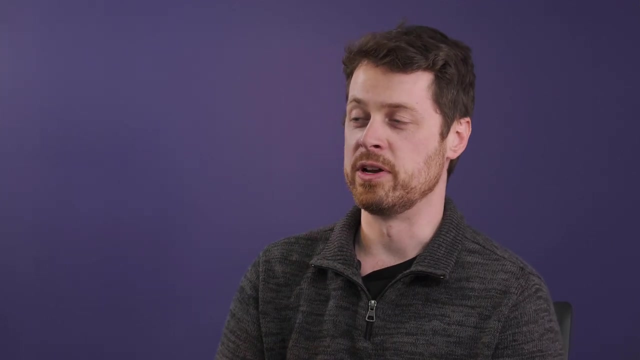 building that up on an optical table is a great way of doing proof of concept testing or looking at the performance of an individual optical subsystem, And when we do those kinds of measurements we have a lot of control over how they're done. So we can look at reducing vibration using a vibration isolating table. We can block out any. 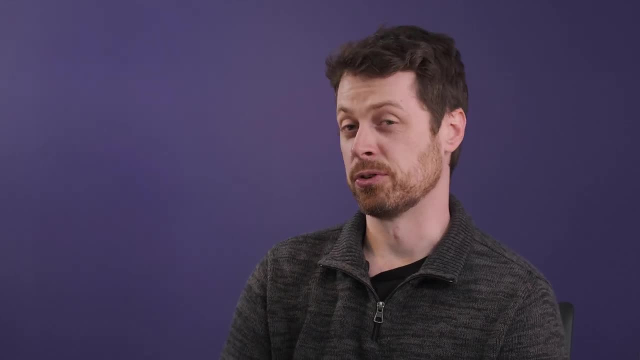 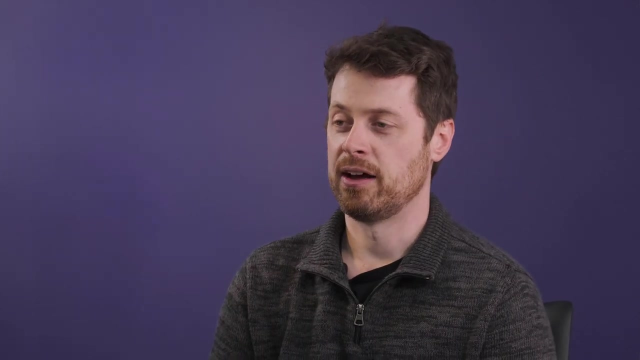 ambient light sources. if we need to, We can control the temperature and humidity in the environment, And we can also keep our optics clean, which often just means not getting them dirty. But as we move into a real medical device, additional considerations become important. 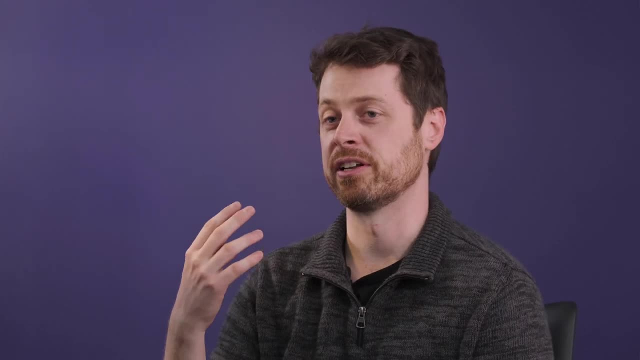 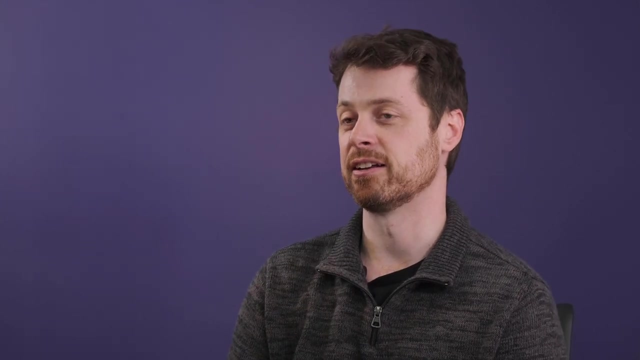 So, first of all, we have to consider how our optical system is going to interact with the rest of the device. We have to think about what the ambient conditions, the ambient light conditions, will be like in the setting where this will be used, and 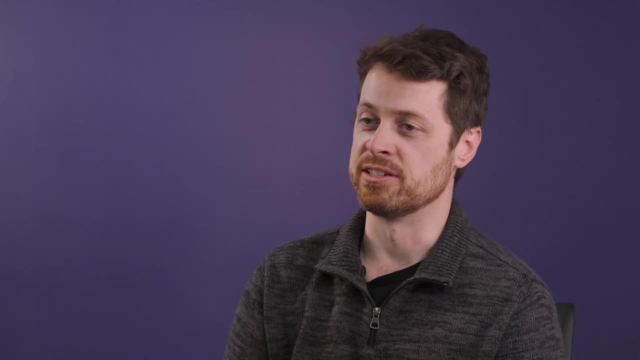 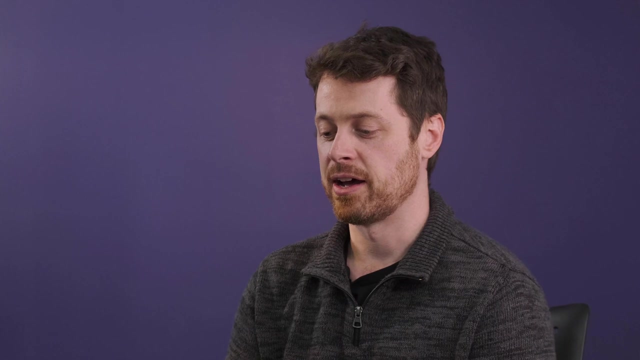 if they'll be variable over time. We need to think about: is this device going to interact with any fluids And, if so, how is that going to affect our measurement? And we also need to think about how we're going to build the device in such a way that it can be kept clean and sterile. 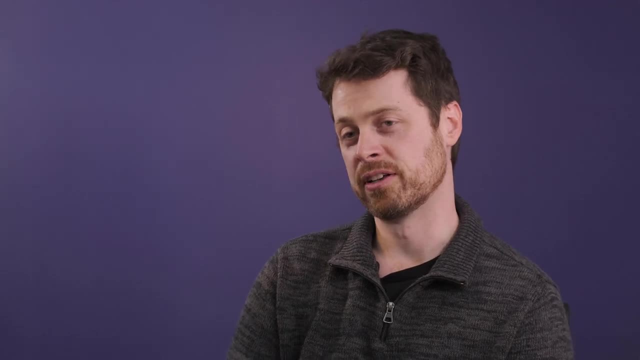 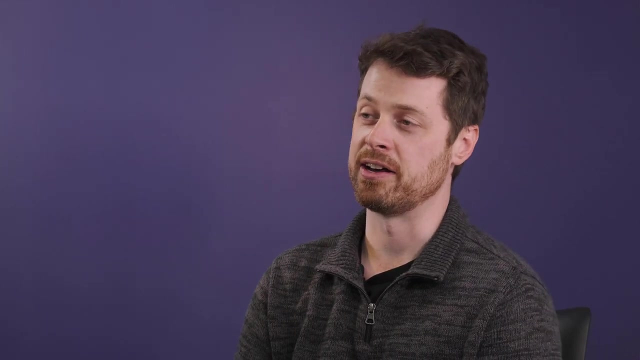 between uses. So when we're doing optical breadboarding, that's a great way of telling us what's possible, But at the same time, we recognize that that's just the first step in terms of testing a device which is eventually going to be used. 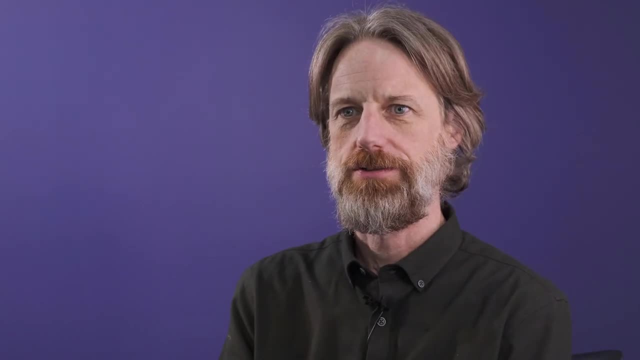 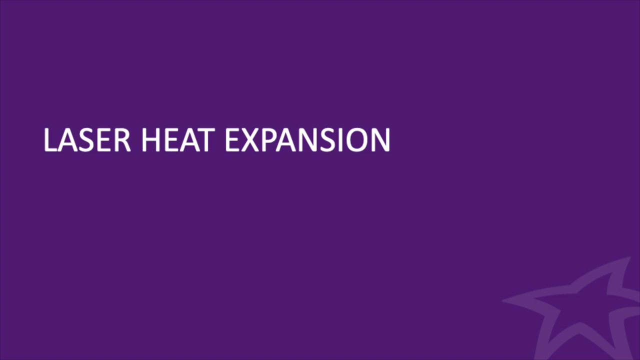 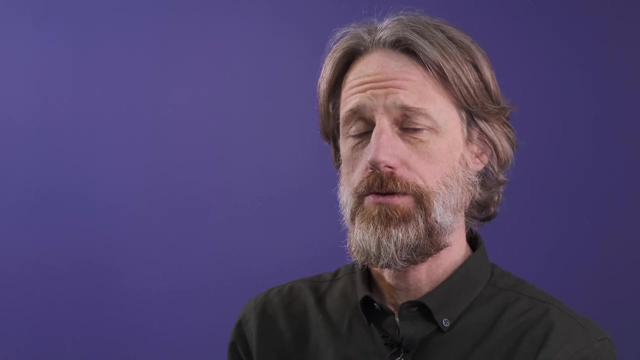 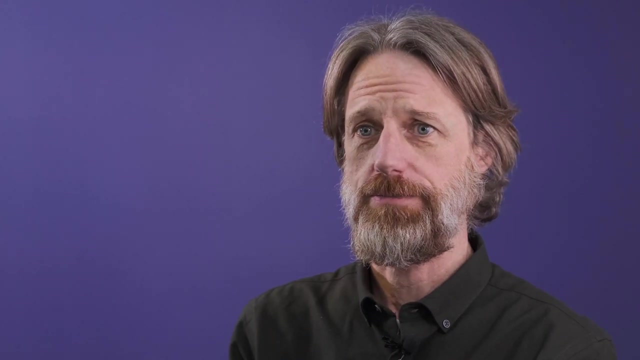 in a clinical setting. My name is Scott Parsons. I work at Starfish Medical. I'm the mechanical engineering team lead for the Toronto office. One of the challenges in mounting lenses is dealing with thermal expansion. The lens itself will typically be a material with high rate of. 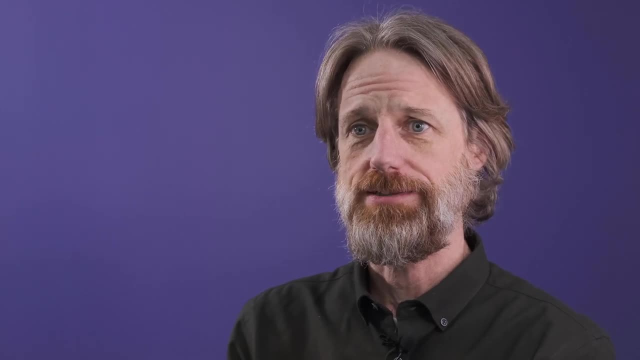 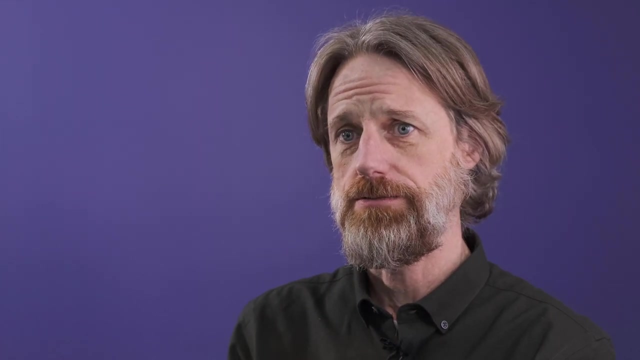 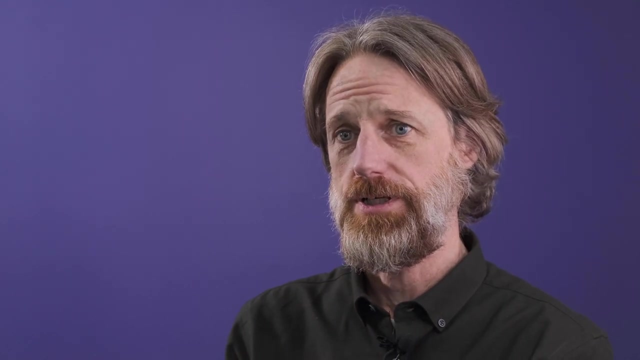 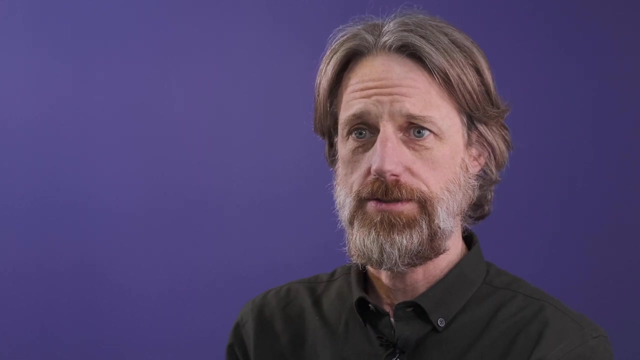 expansion Thermally Something like glass, The mount will have a lower rate of expansion, being steel, aluminum or invar. Invar is a material that's used in optics because of its low rate of expansion over the heat range. The problem that is faced is when the outside mount is made of low. 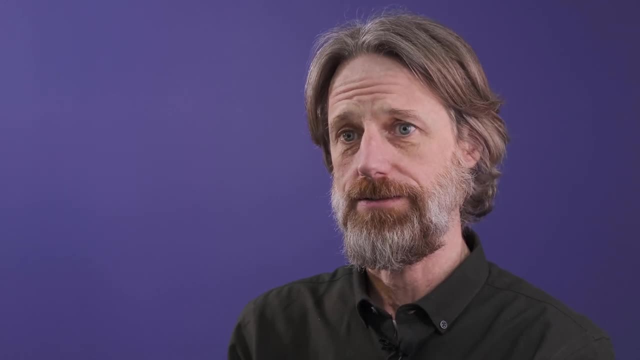 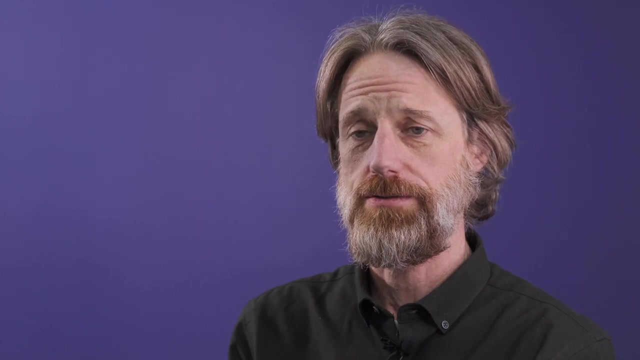 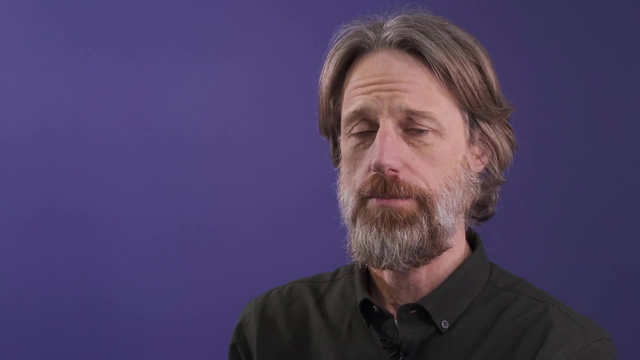 expansion material and the glass is expanding faster. When heated up, there's the potential for the glass to expand beyond the mount and crack. The design solution for this is by creating a proper gap between the lens and the mount. This is achieved with the adhesive gap between the two. 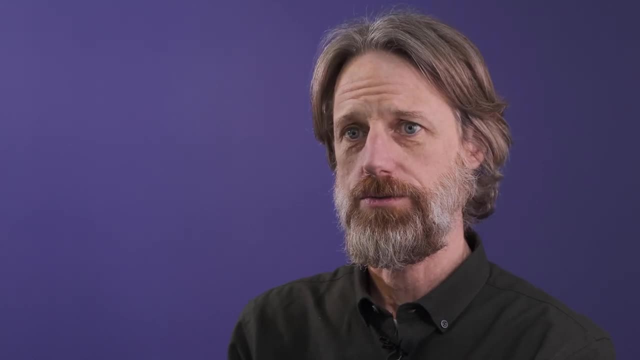 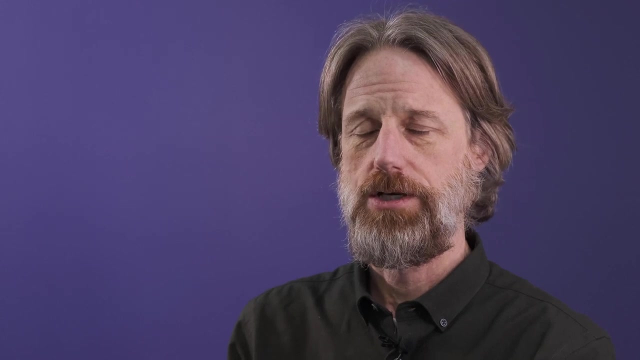 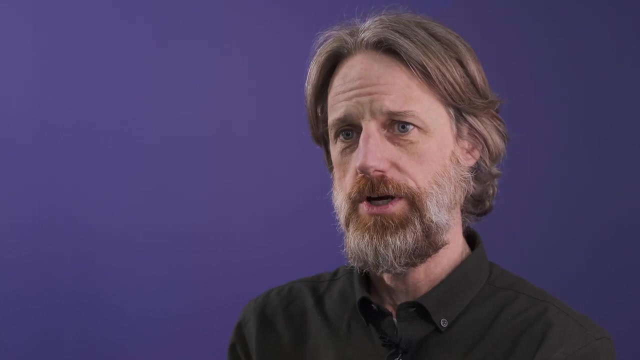 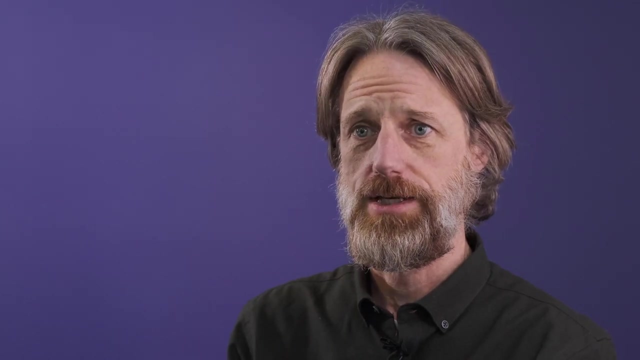 In looking at this adhesive gap. it is important to to maintain the distance so that we would never have a situation that where the lens cracks, but also considering the relative stiffness of the system. If vibration isn't introduced. we do not want resonance to occur with that adhesive and the 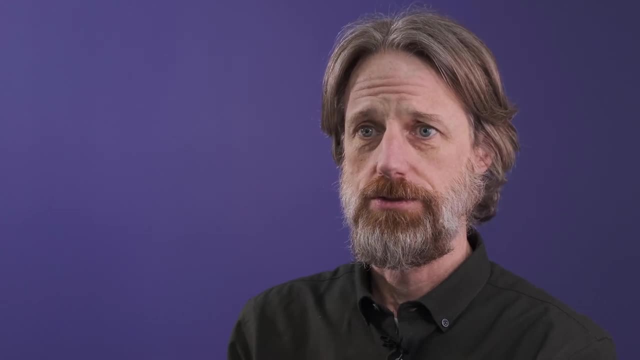 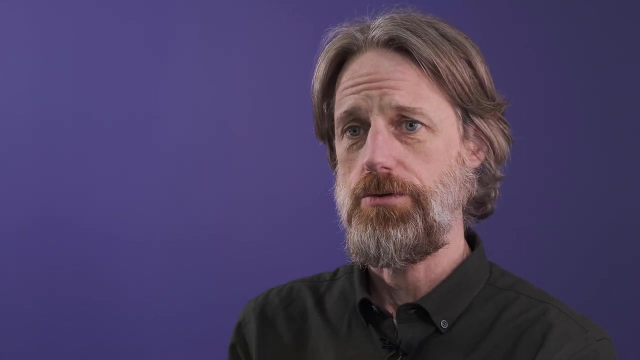 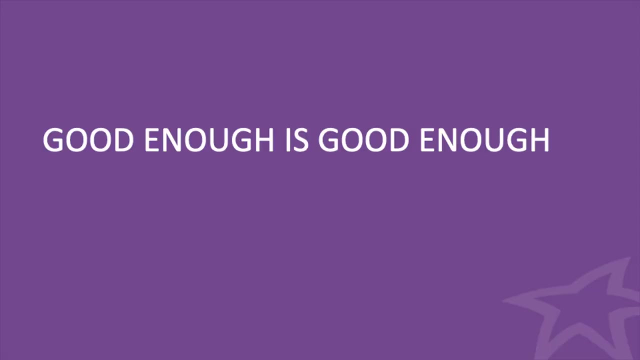 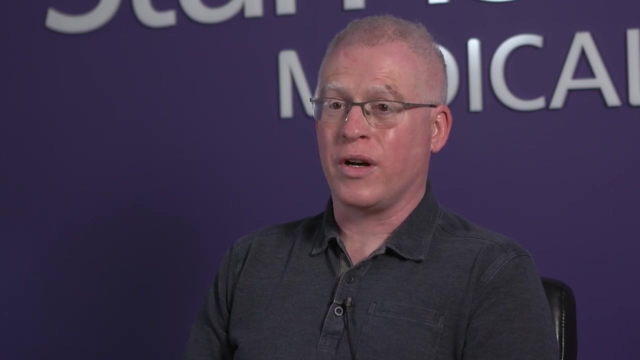 lens and thereby shaking the image. So calculations need to be done to maintain the proper stiffness of this, but also ensuring that we have room to grow throughout the temperature range. An important thing to remember when approaching an optical system design is that good enough is. 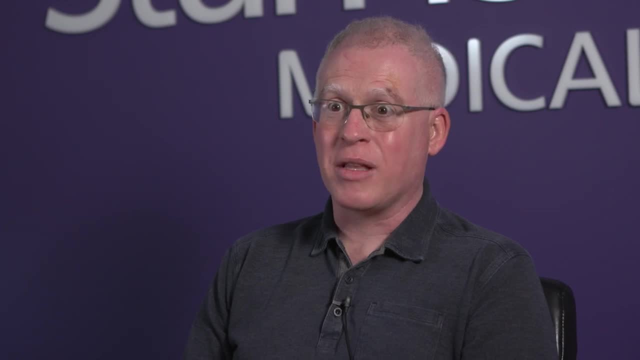 good enough. Sometimes there can be a temptation to design the perfect optical system or the perfect measurement system, but you need to keep in mind what your requirements are and do sufficient engineering and design to reach those requirements And give yourself a little bit of tolerance margin, but not spend unnecessary time and effort designing.